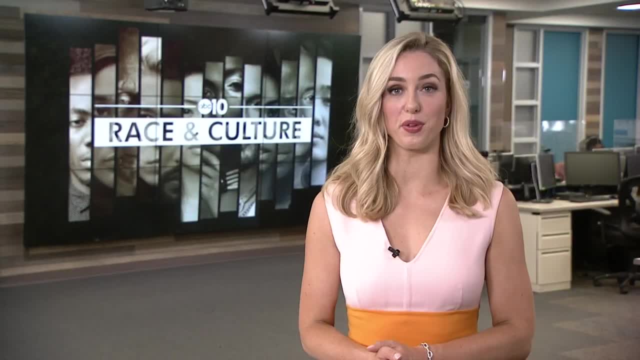 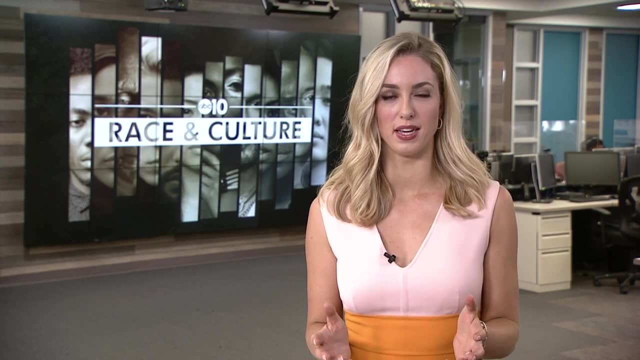 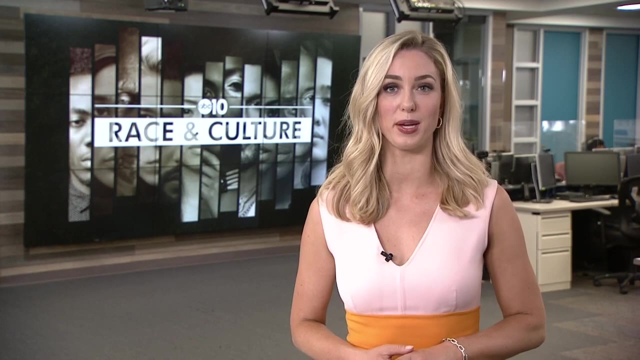 The CDC says gun violence in the US increased about 35% during the pandemic. That's the highest level since 1994.. Even though gun violence impacts all communities, black people and those living in poverty suffer the most. Tonight, ABC 10's lead race and culture reporter, Candace Redd, explains why. 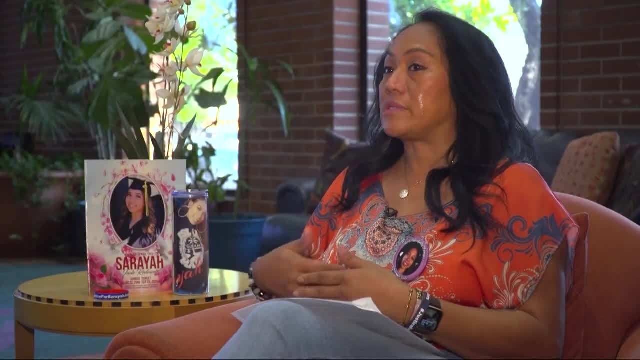 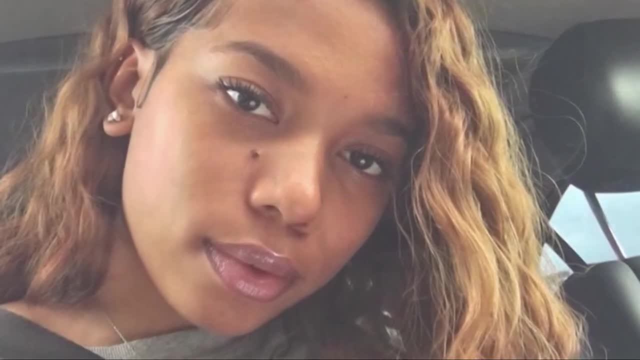 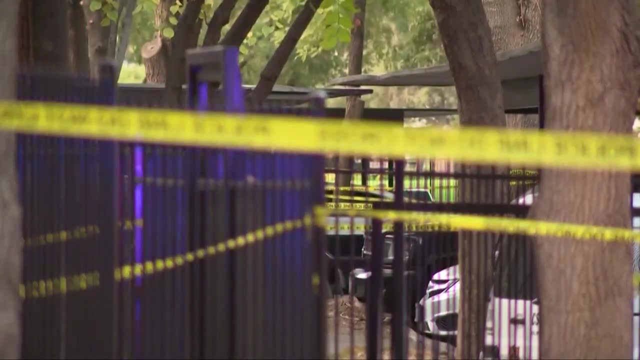 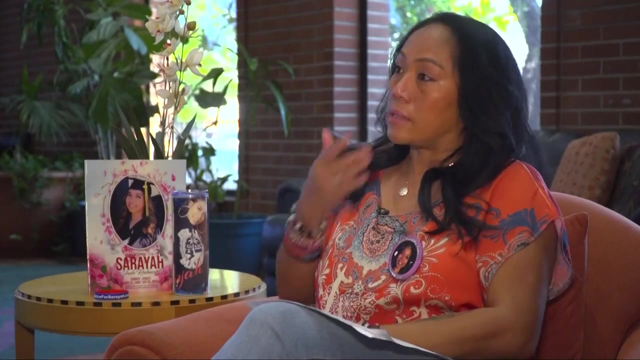 You know I have to be her voice, because if I'm not her voice, she'll become forgotten. Jennifer Redman continues to fight for justice after the loss of her 19-year-old daughter. Police say someone shot and killed Soraya Redman at the Stone Creek apartment complex in Natomas on September 25th 2020.. I can just imagine her screaming and the sad thing is like nobody has said anything. 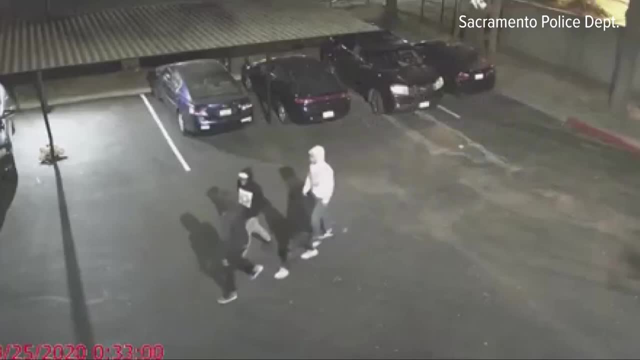 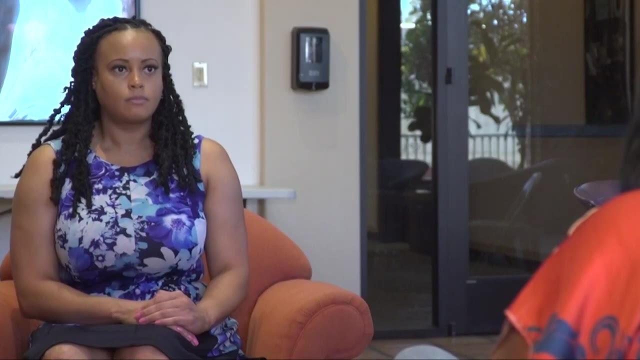 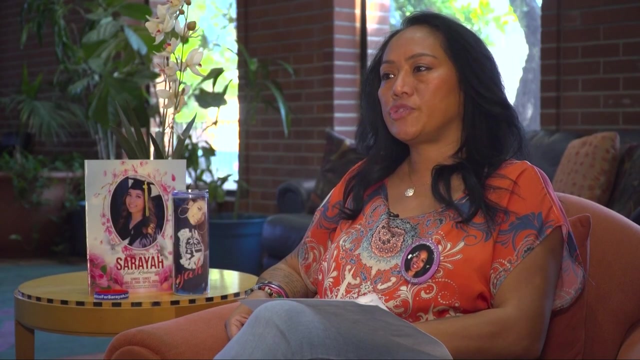 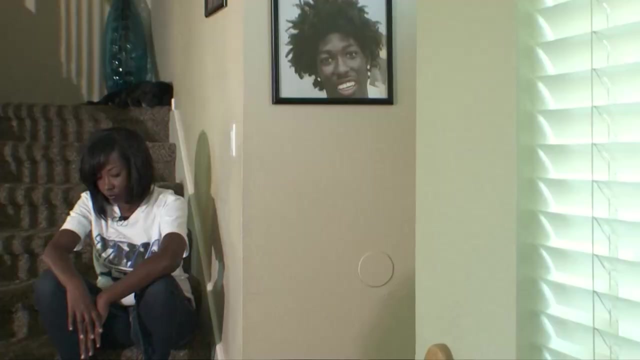 Police released this video, This surveillance footage, last year in April showing a group of people possibly connected to the crime. To this day, the case remains unsolved. My fear was always what could happen to my sons because they were black men. I never thought I'd have to worry about my black daughter. I don't want no other parent to go through what I'm going through. 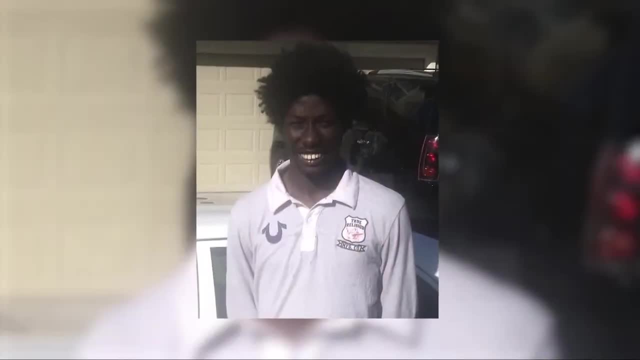 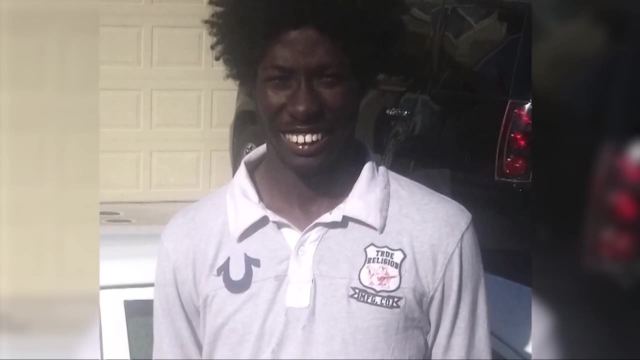 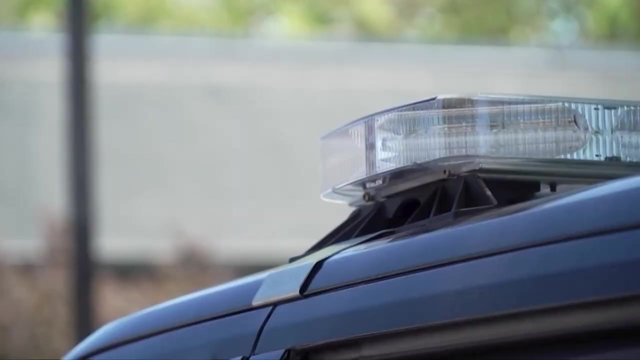 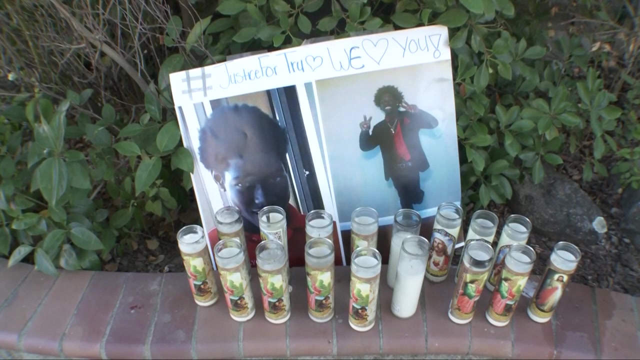 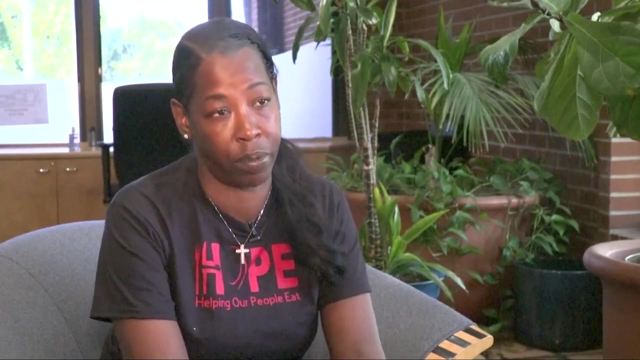 Eugenia Whiteside is a heartbroken mother too. She says someone shot and killed her son, 17-year-old Deonta. She says someone shot and killed her son, 17-year-old Deonta Whiteside, in front of their home in Elk Grove on June 23rd 2016.. Sometimes I wonder, before things happen, like with my son, that they think about the effect it would have on me. Police arrested and charged a group of six people in connection to the crime. They shot a little girl after they shot my son to cover up his murder. She lived and so she was able to give them information that they needed to arrest the people. Even though all communities face gun violence, some suffer more than others. The CDC says. 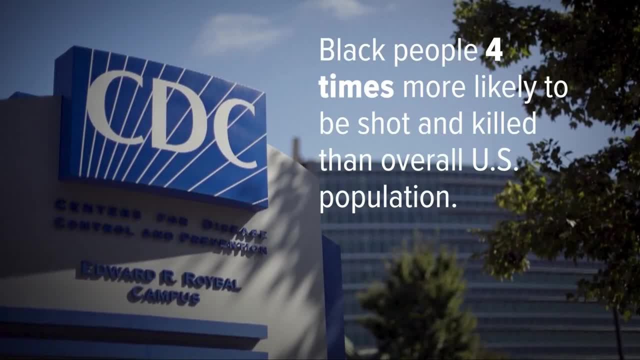 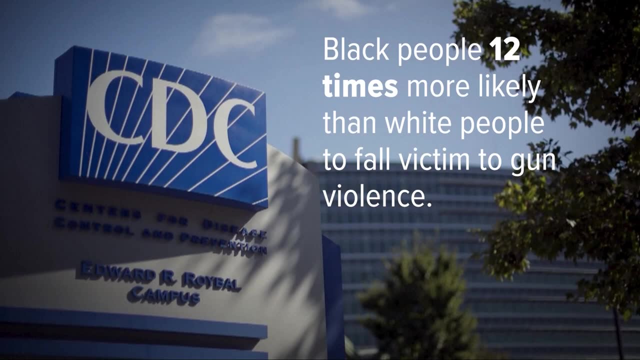 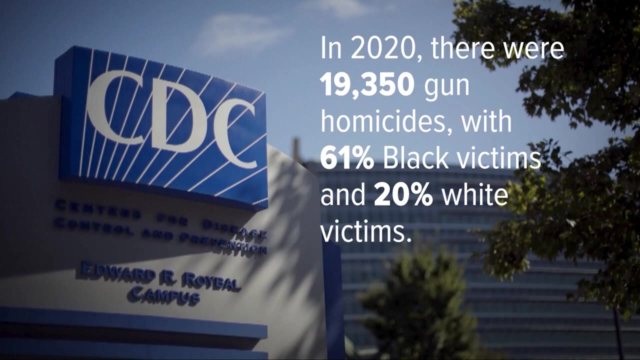 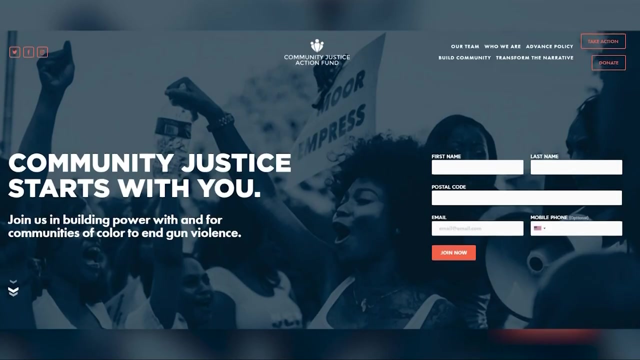 black people are at least four times more likely to be shot and killed than the overall US population. They're also 12 times more likely than white people to fall victim to gun violence. In 2020, there were more than 19,000 gun homicides, with black people accounting for 61 percent and white people 20 percent. Our country has failed to look at this as a public health crisis. Gregory Jackson, who's with the Community Justice Action Fund, says racial disparities and gun violence exist, but